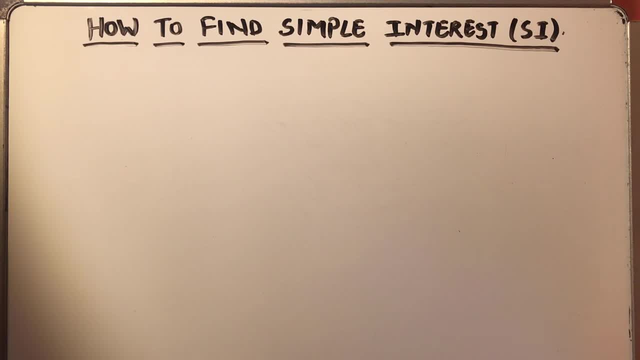 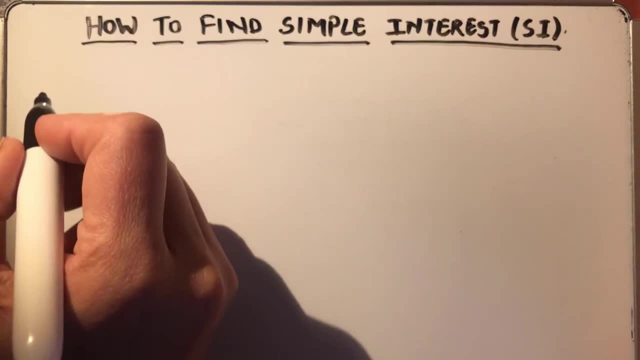 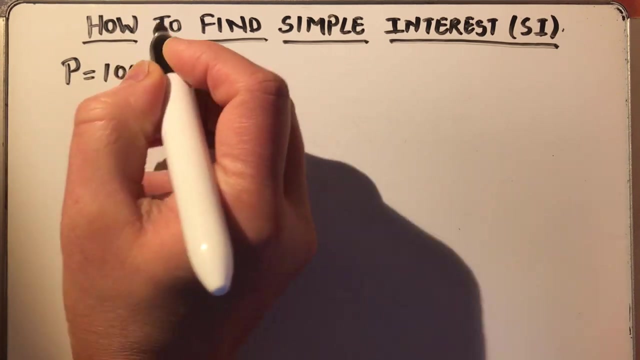 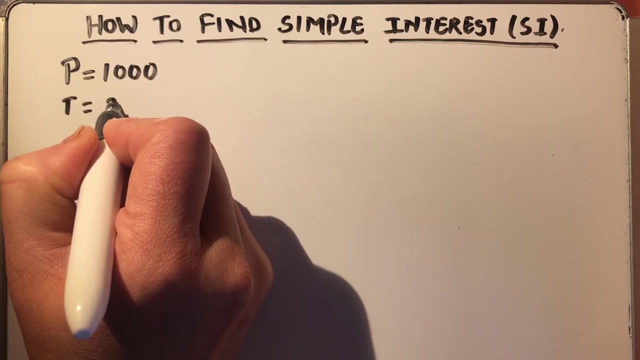 particular rate of interest. that is called the. that amount is called the simple interest. so let's see how we calculate that. so too, for suppose we have taken a loan from a bank of rupees, thousand, thousand rupees, loan we have taken, and we have taken the loan for two years, and the rate of interest, the rate. 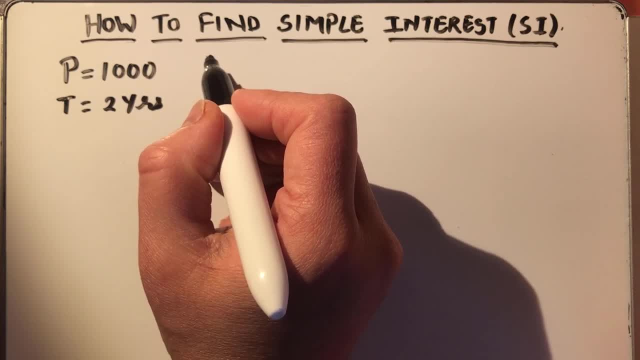 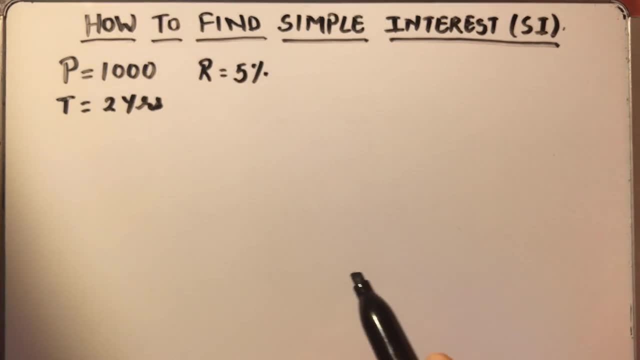 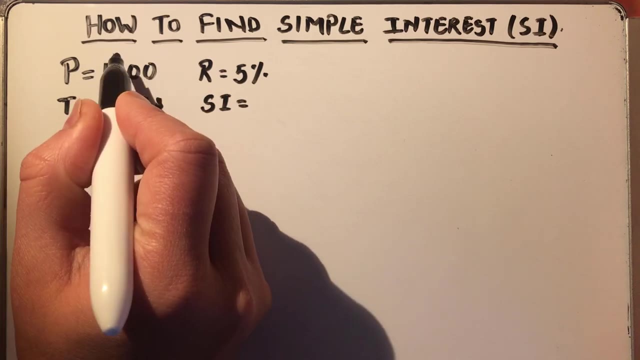 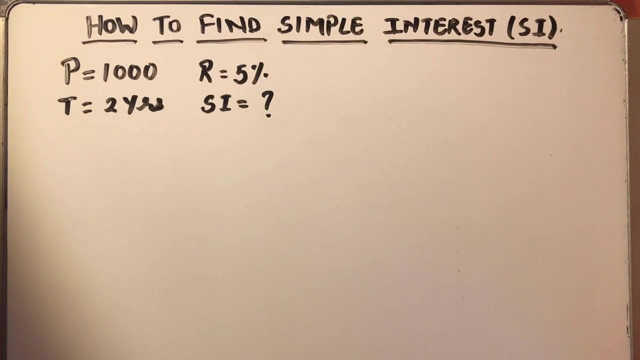 of interest is the interest the bank charges on this amount. so let's see, it is 5%. so we need to find the simple interest, the amount which we need to pay extra. apart from this amount, we have to pay some extra after two years. so that is called simple interest. there is also one more interest. 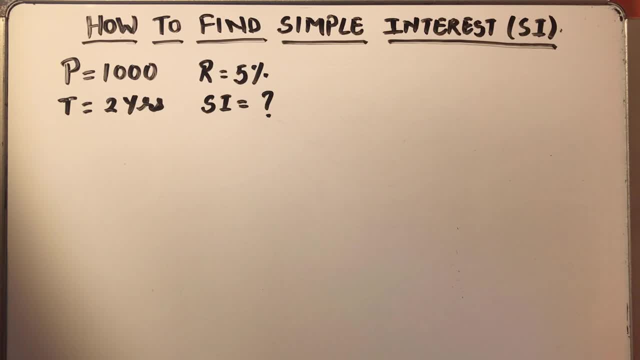 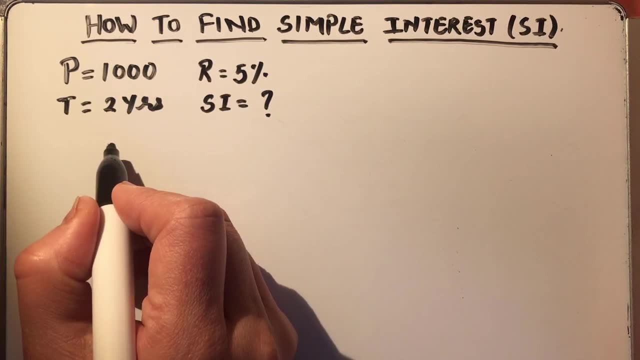 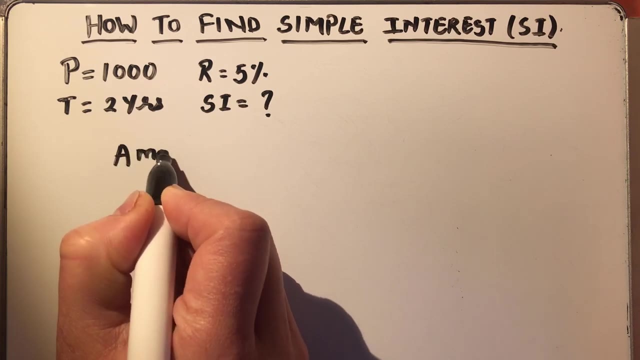 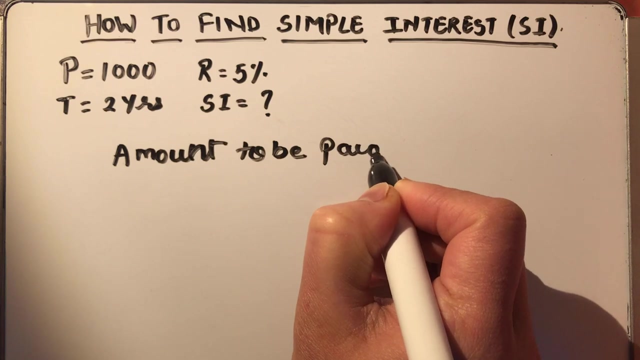 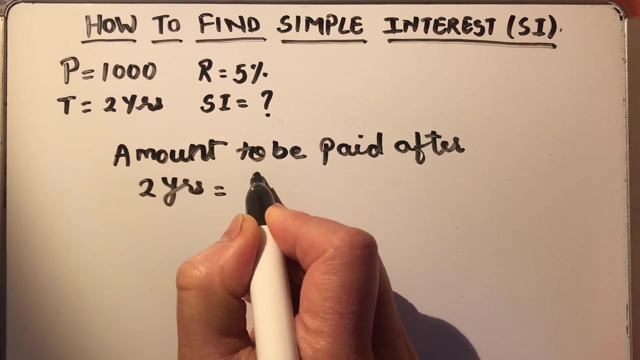 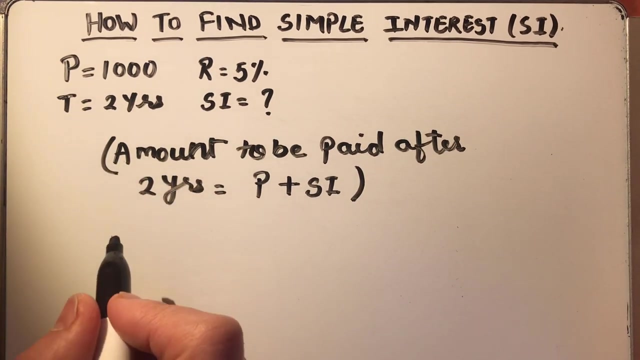 which is called compound interest, and I am going to upload a separate video for that. first we learn simple interest. so to find simple interest, So our amount to be paid after 2 years will be will be principal amount plus simple interest. Okay, now let's see how we calculate simple interest. 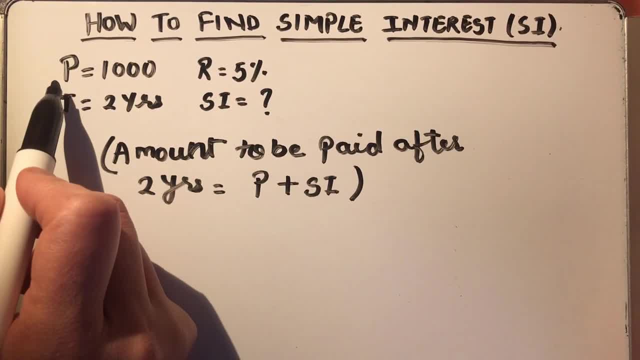 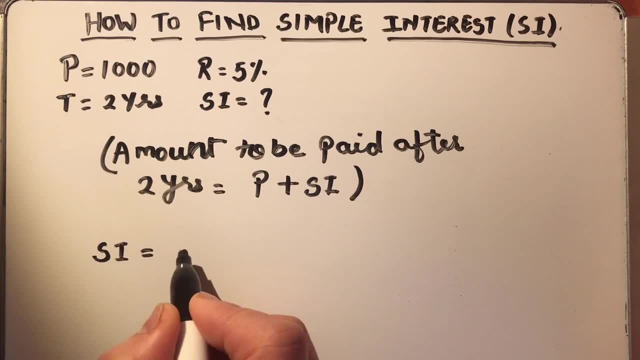 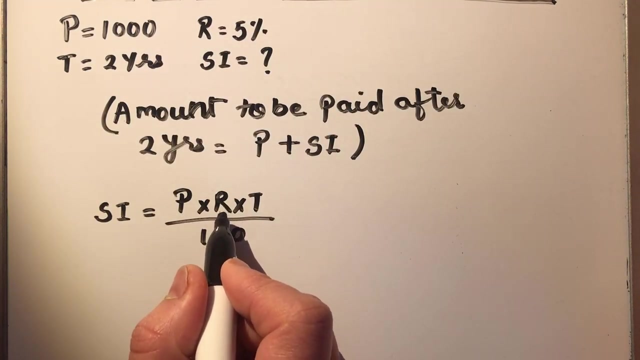 So I will be writing SI for simple interest and principal for the amount for the loan we have taken. So simple interest is equal to P times R, times T over 100. So where P is equal to principal amount, R is the rate of interest which is yearly. 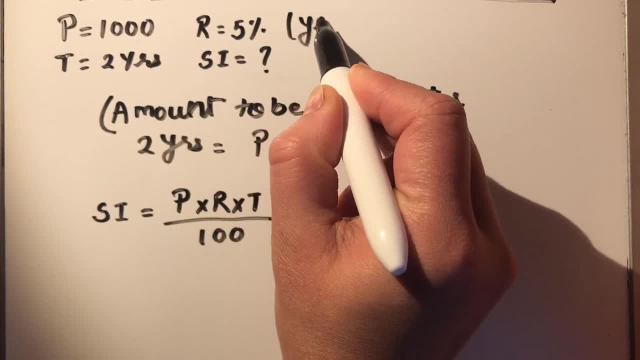 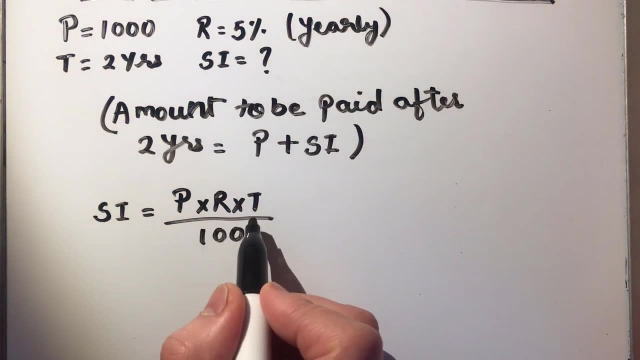 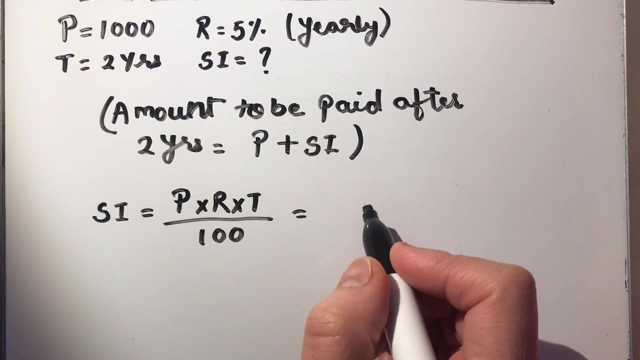 Okay, Rate of interest. here we are talking about the yearly rate of interest For 1 year. they will charge 5%. So this is R, T is the time period, and over 100.. So let's put the values here in the formula.